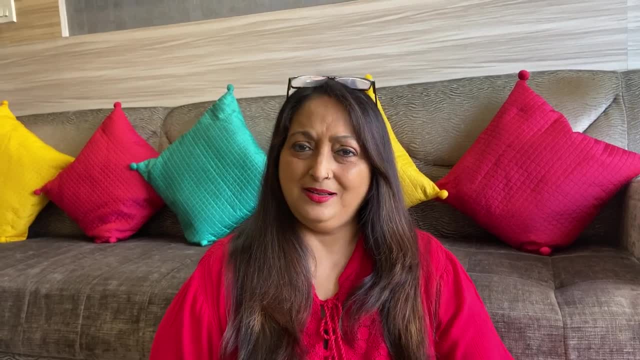 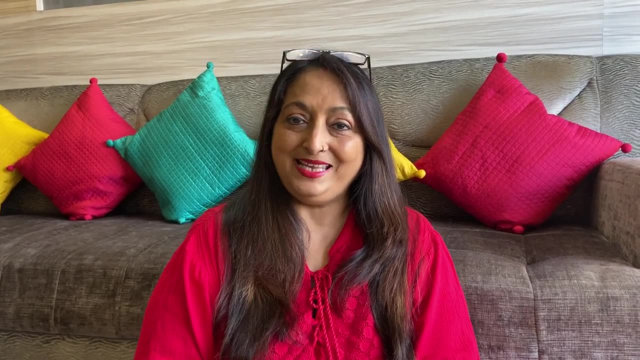 And you need a rolling pin along with that, and you need a cutter just to cut out the gift shapes. That's all that you need for the first part of the activity. Now for the second part of the activity. what do we need? We need some cutters. 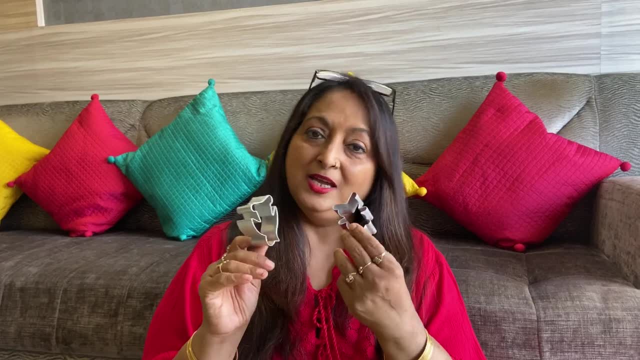 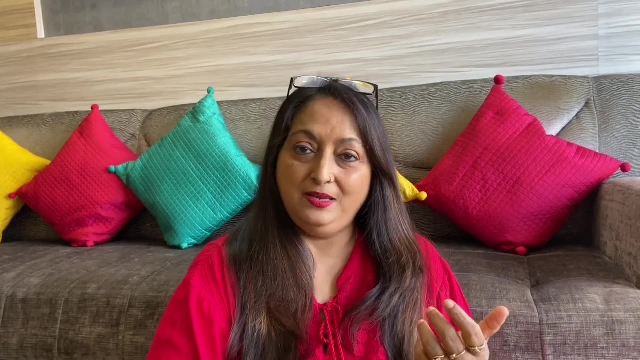 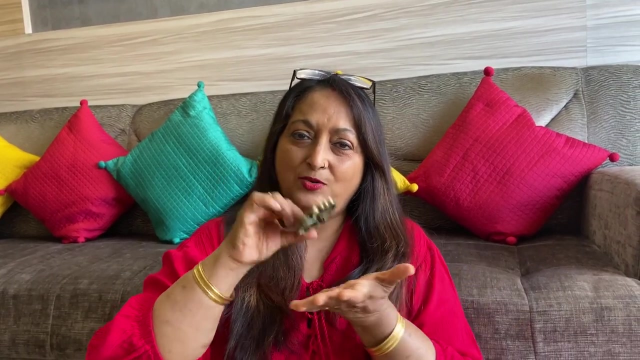 You can take any cookie cutters. if you don't have, You can take your glass or a board or anything. And we need certain things to make an impression. So we can use a fork, we can use a key, anything that you find around the house where you can press it down and form an impression. 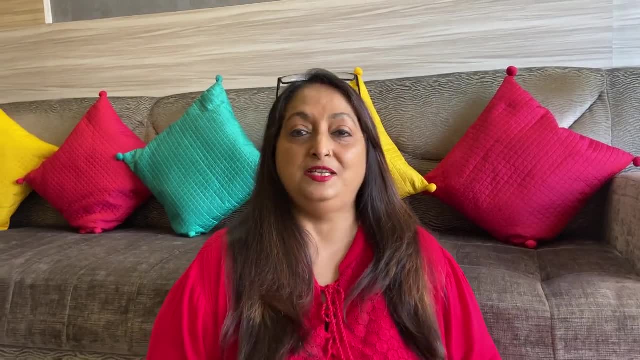 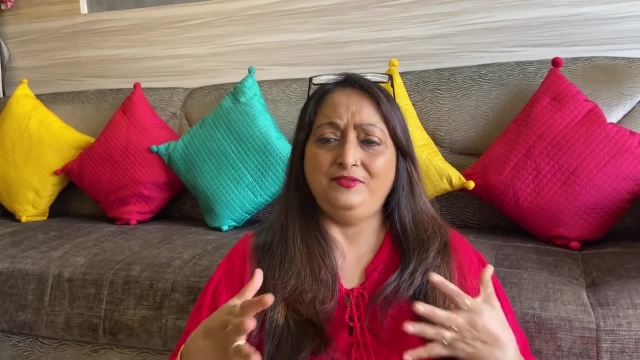 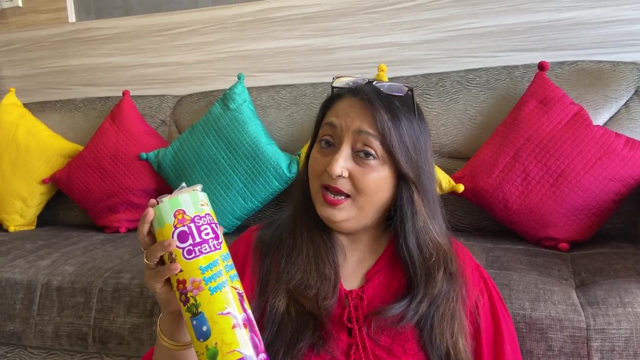 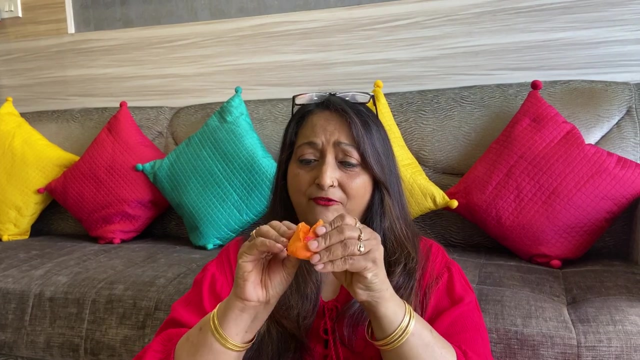 Now this is a very good activity for the children, for their muscular movement, for their gross motor movement, for their creativity, And it can be done with any of these things. I have bought dough set and it says that it is super light, super elastic and super bright, and it was super bad because it was like rubber, like foam and it was horrible. 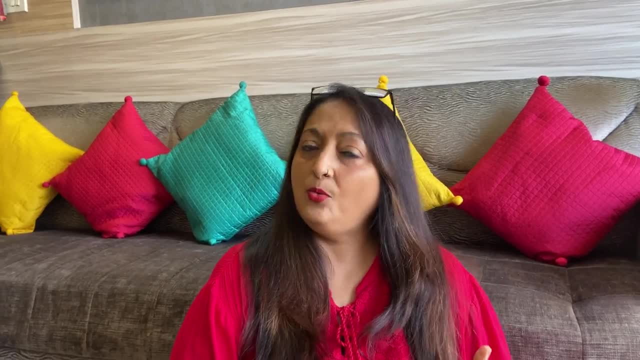 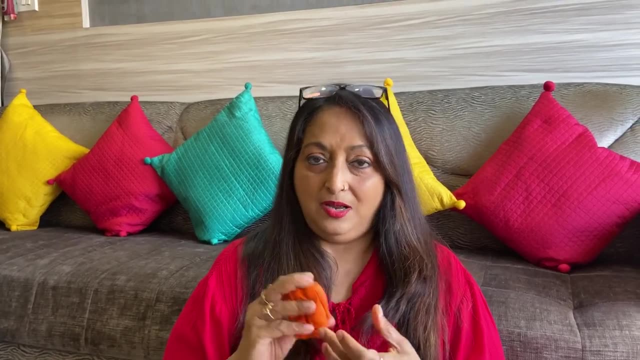 So what I did? I made my own dough. So I took some water color and I took some refined flour and I made this dough with that water color and flour, make it at home. and the trick is, after you made it and your child is played. 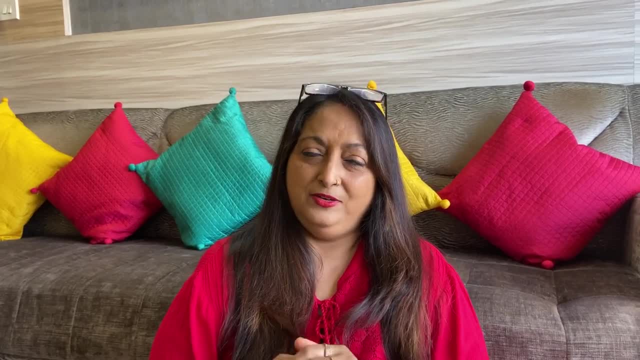 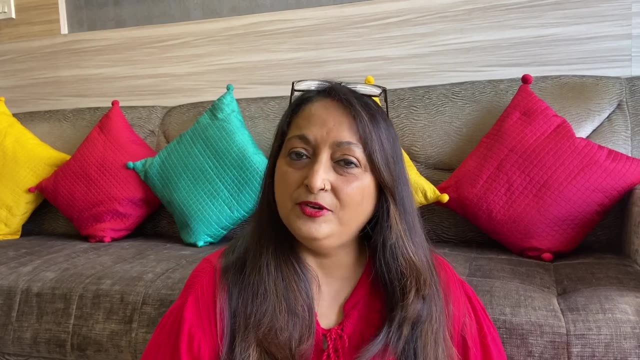 with it. just put a little oil and put it, you know, inside, cover it up with the foil paper and refrigerate it, keep it in the fridge and whenever you need it you take it out. I think it lasts you for about a week, before it's get before it. 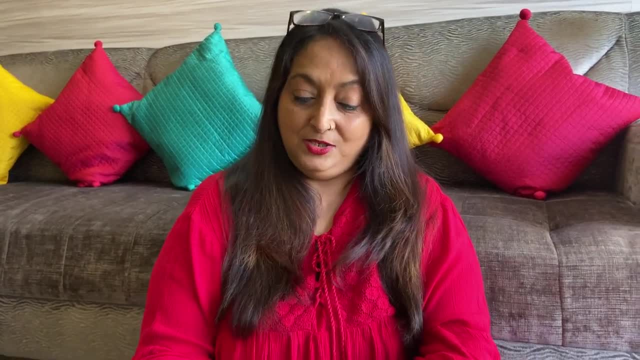 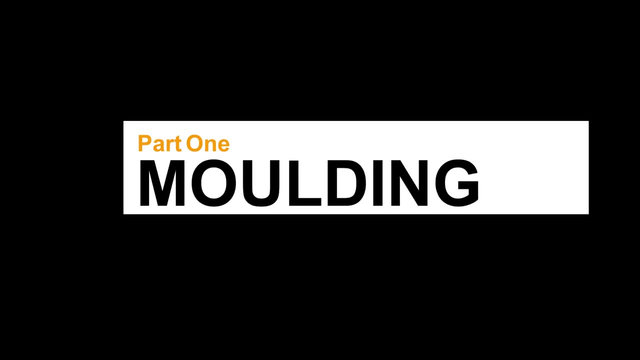 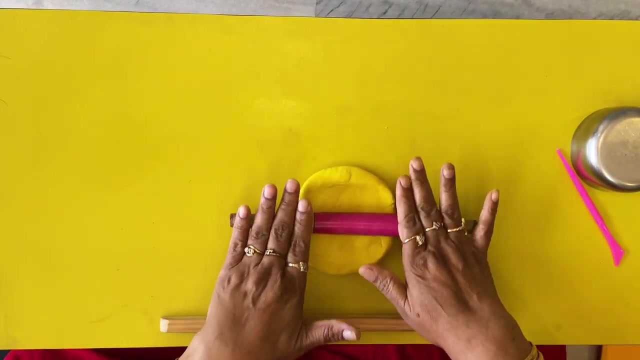 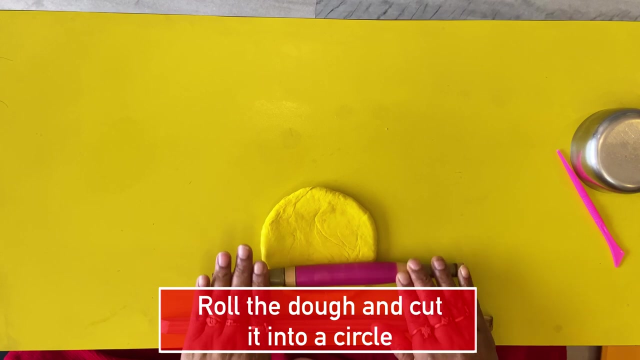 gets bad. so you can do this in the house. so let's get started with the activity. so let's take some yellow dough and roll it out, and then we are going to cut it in a circle shape. I don't have a circular cutter, so I'm going to use a 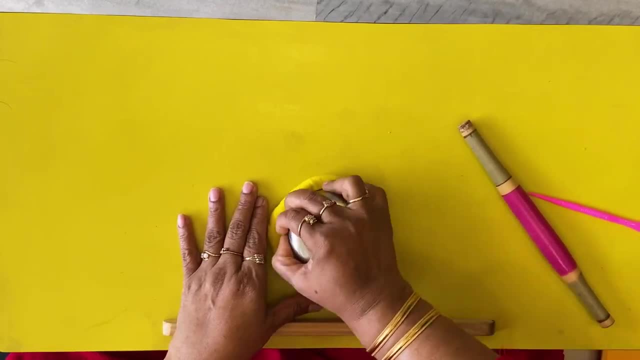 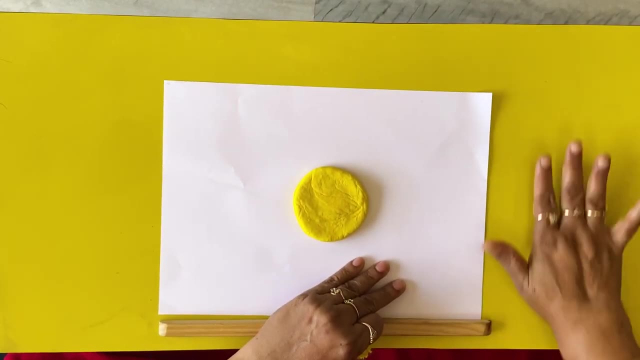 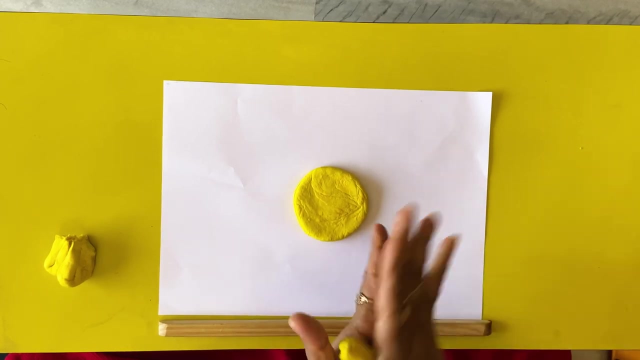 bowl. you need to press the ball hard and here we have the circle. now we are going to make a Sun. so what is the next thing we need to do? we need to make the Sun's rays, and we can continue to make the rest. now, this is a very easy thing for the children to make. parents can help them, they can do. 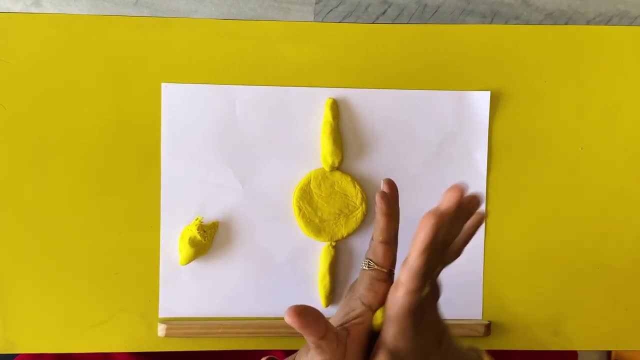 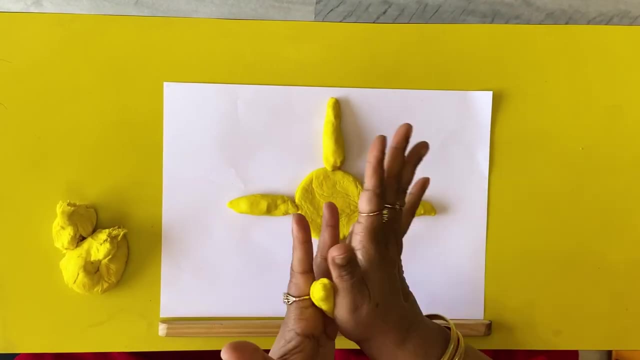 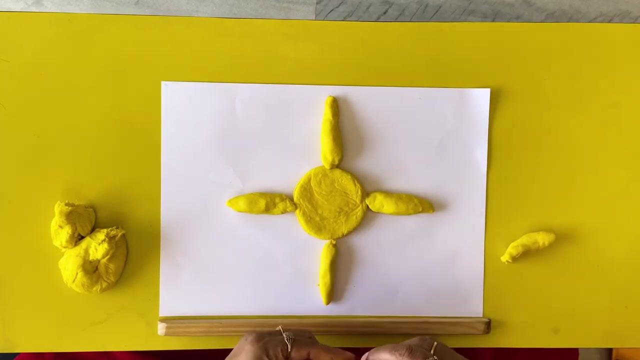 this within their palms, between their palms, or they can roll it on the table. they can do anything and this is an excellent gross motor exercise for the children. this is going to increase in creativity. they may want to make different things more, something different, different from what you are telling them. it doesn't. 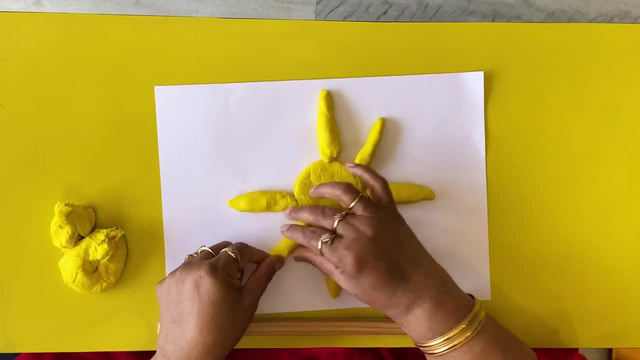 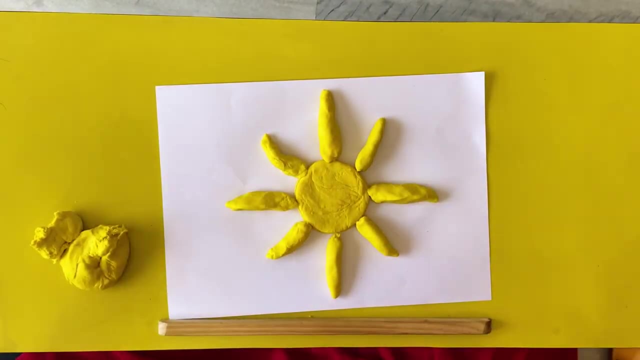 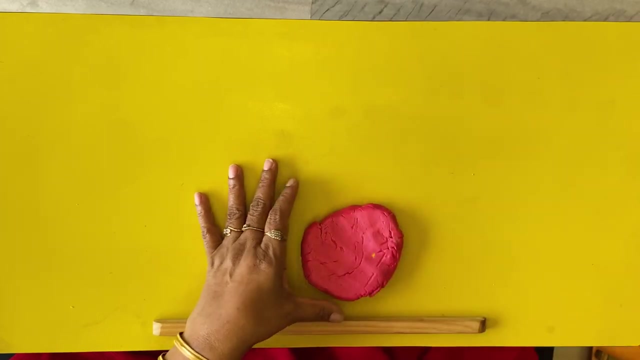 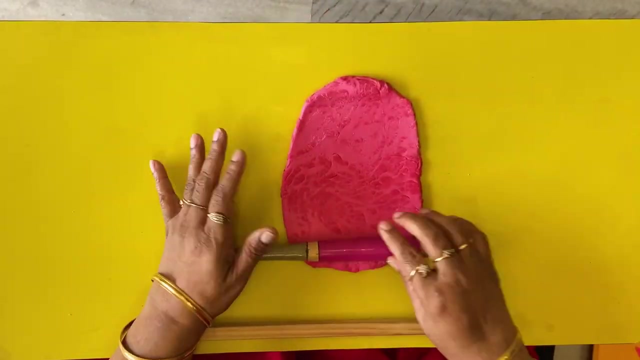 matter. it may not even look like what they are saying, but just being creative. creative is good enough. now this is a Sun, so hope you liked it. let's take pink dough. so what do you think we can do with the pink dough? with the pink dough, we are going to cut out small circles and we are going to make it into a 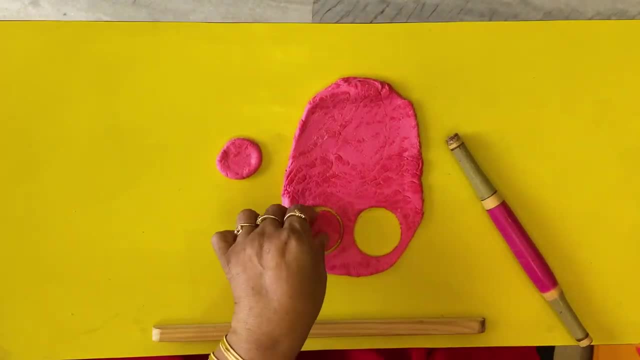 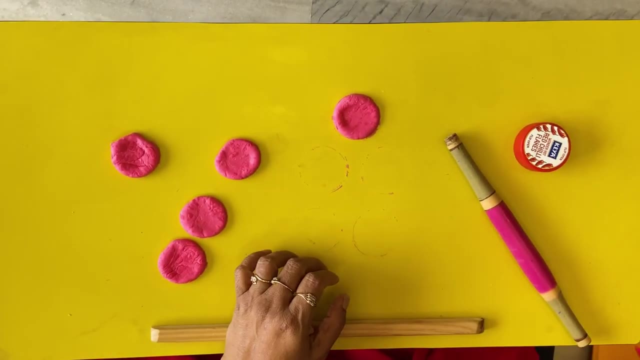 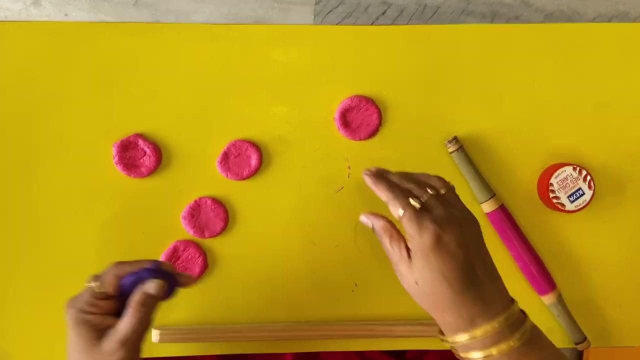 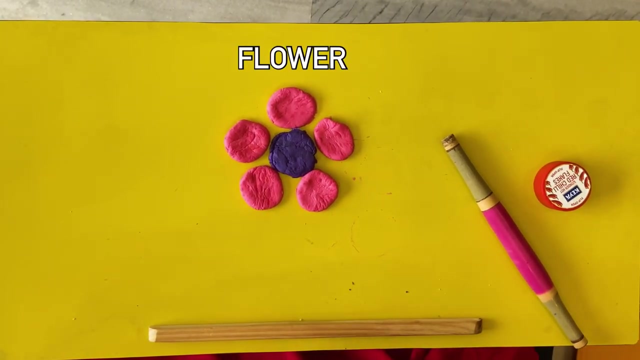 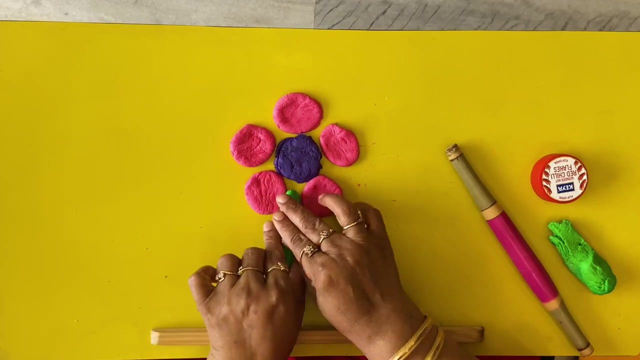 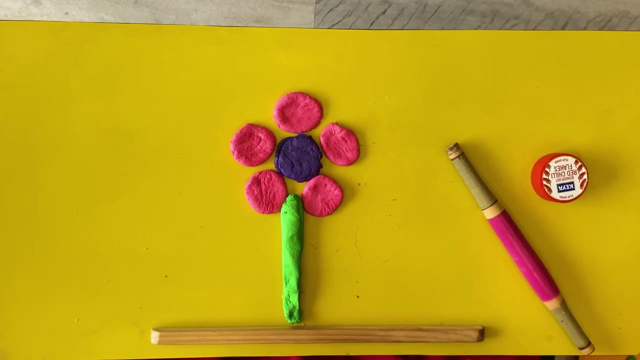 flower. I think this looks beautiful. but now we need to make the stem and believe so let's do loud, some green door for the stem and just place it. now we need the leaf. now we can just press the leaf between our fingers just to give it a shape, and then we're going to cut it. not cut it, just give. 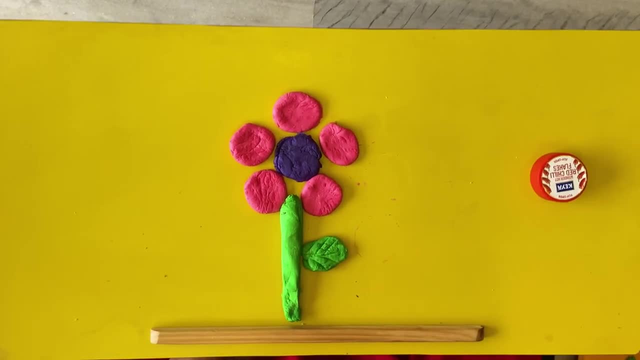 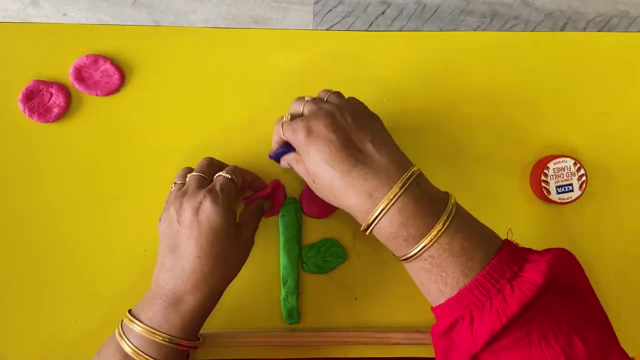 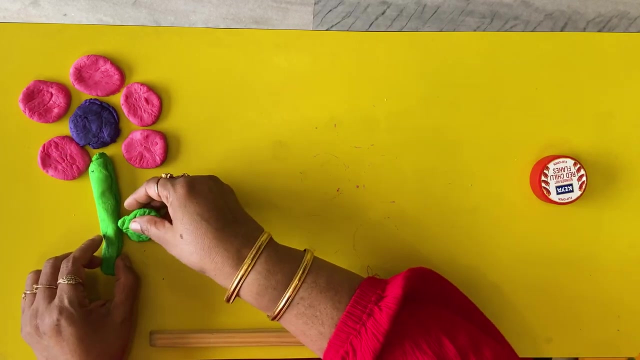 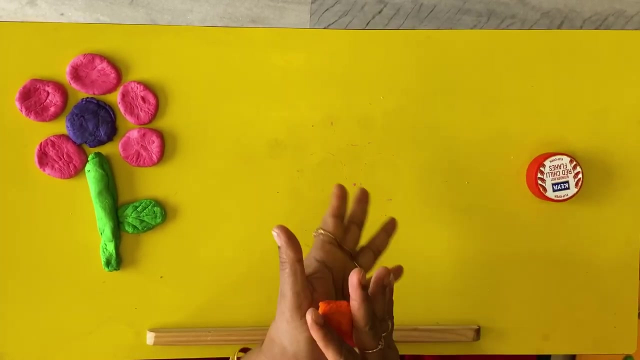 it portions of the leaf. so, wow, that's a beautiful flower. now let's make something else so we can just shift this flower this side- it's very easy to shift it also here. and let's do the next item. i think i'm going to make an ice cream- corn ice cream. 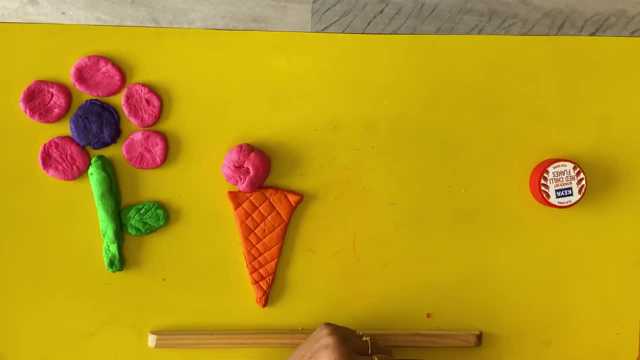 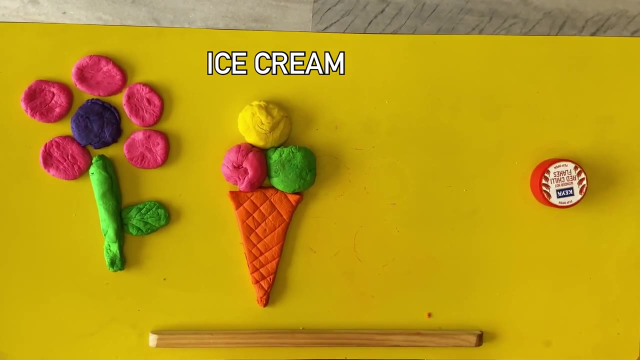 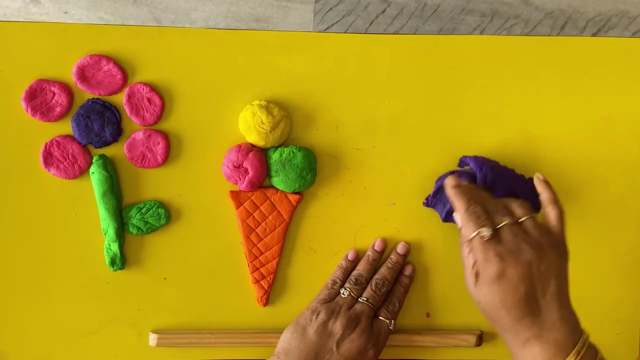 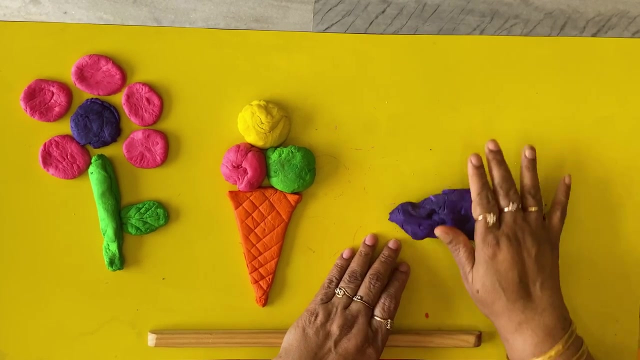 so, wow, delicious ice cream is ready, and i'll make one more thing for you. the last thing: so i have a lot of purple dough left, so what do i do with purple dough? can you think of something we can make with purple dough? so let's start and let me see if you can guess what i'm making. 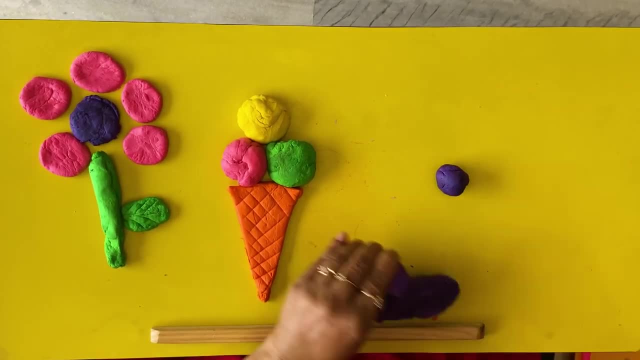 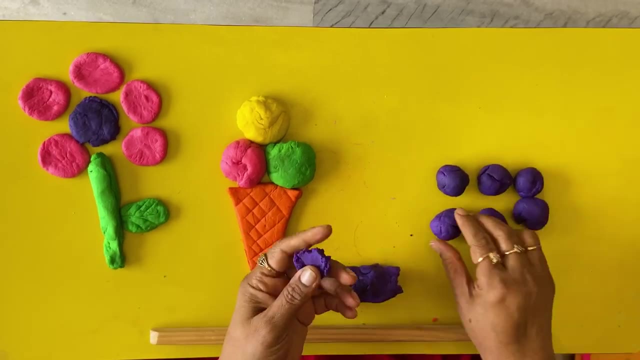 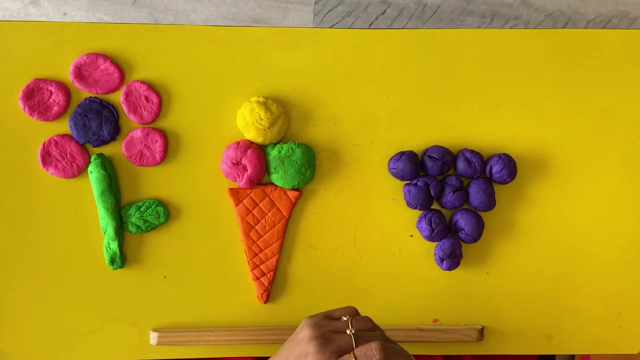 are. children of any age can do this, whether he's like one year or five years or eight years. children would love to do this. they love to be creative. so here we are done so let your children do this. they're going to have a lot of fun. 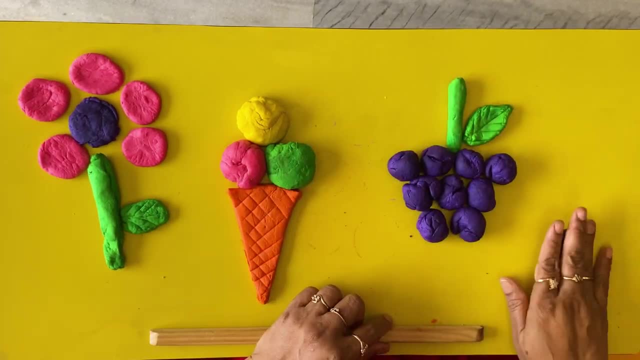 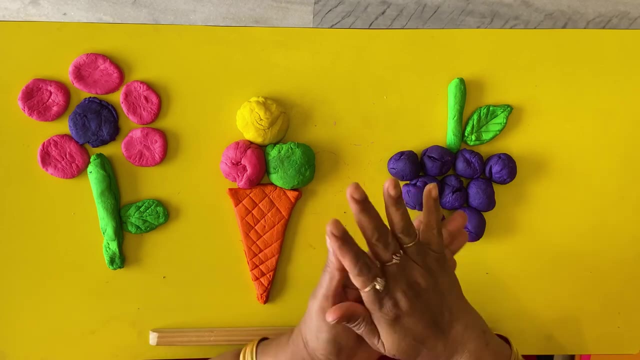 and this is an excellent exercise for the children- all gross motor movement. all this doing this, it's really good. the muscles of the hands are going to strengthen and they'll be able to hold a pencil, a crayon properly and write, so this is extremely important. this is a very useful activity and it's also very 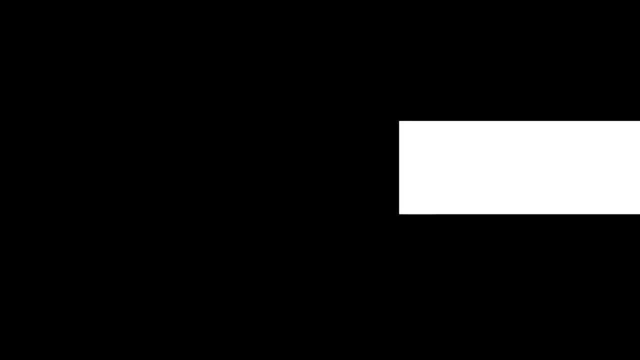 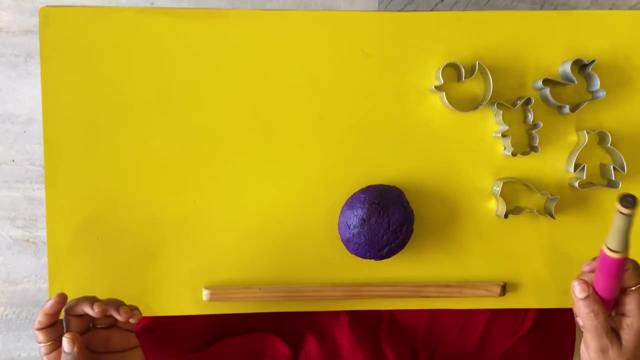 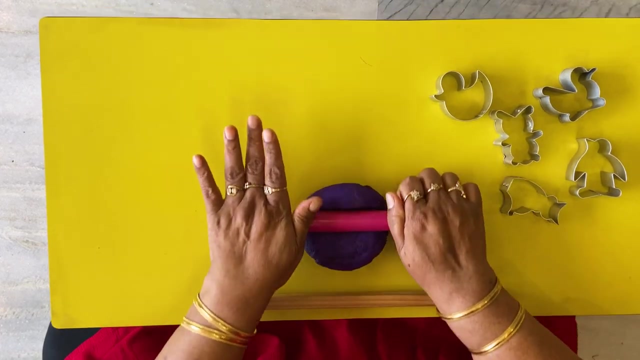 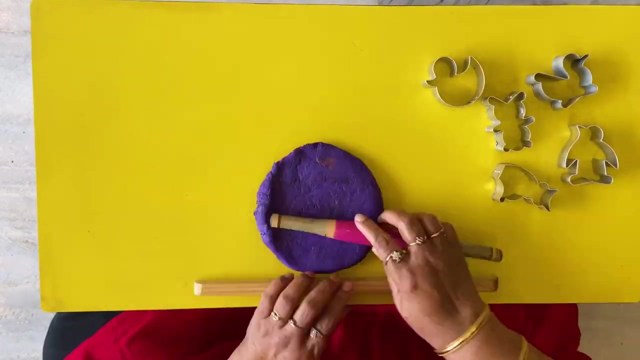 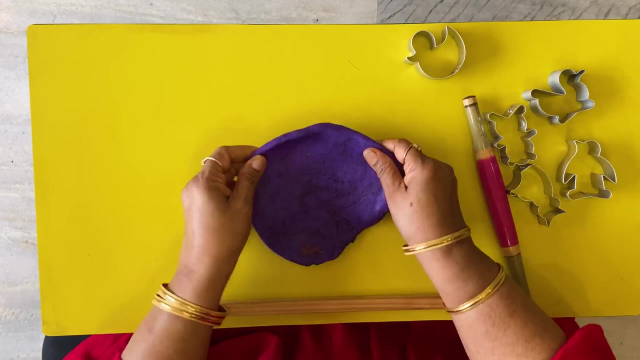 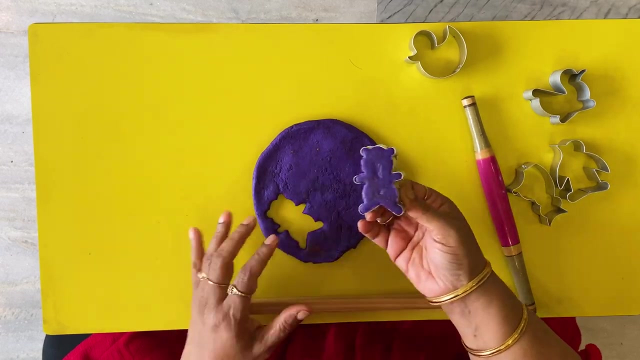 creative. now for the second part of this activity. we are going to take a dough- any dough you want- and we're going to roll the dough, press it hard. only then it's going to cut. this has just come through. push it and we have a pretty little ball. 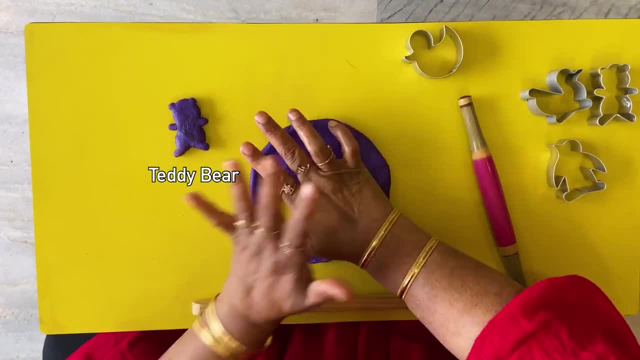 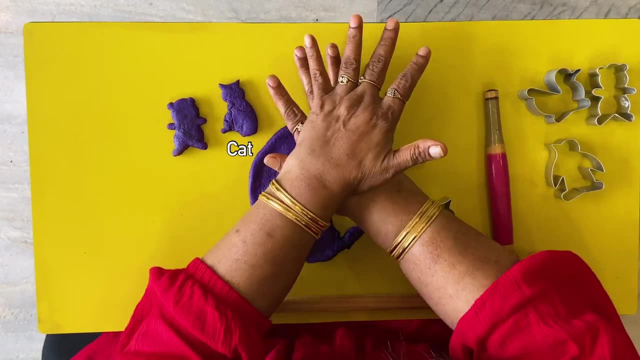 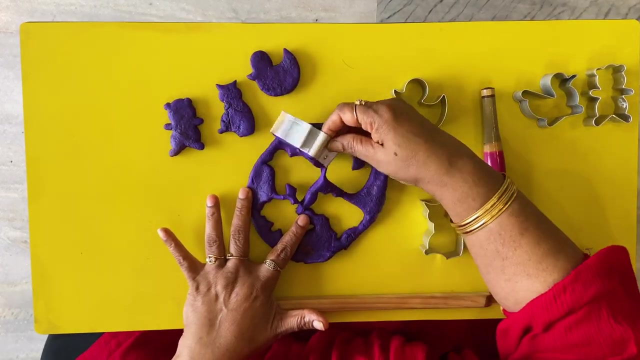 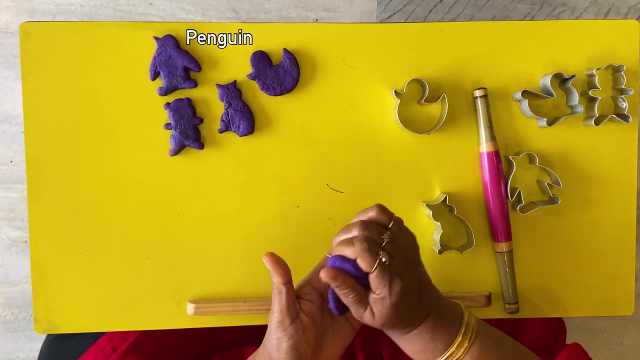 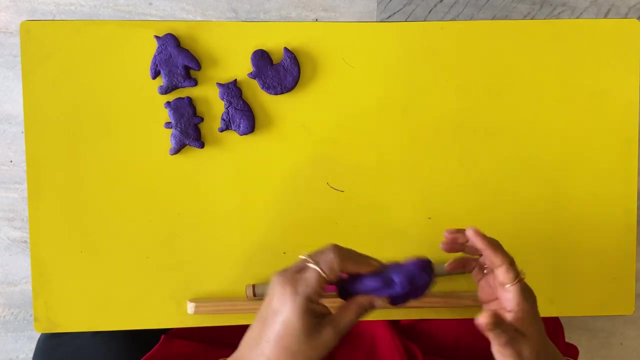 teddy bear. I'm going to apply force so that they can make stronger strokes while writing. so here we have the penguin. so this is really pretty. so we remove these cutters. and what else can we do now? let's see. so we are going to take another color, so 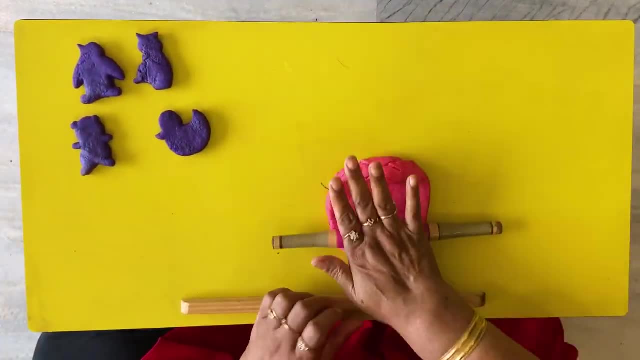 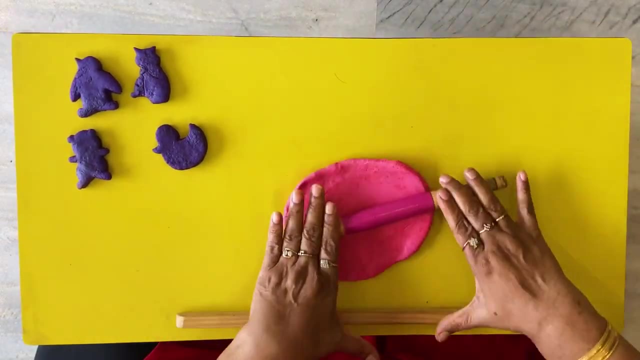 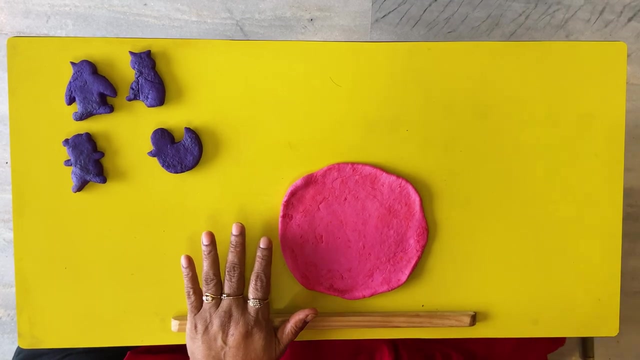 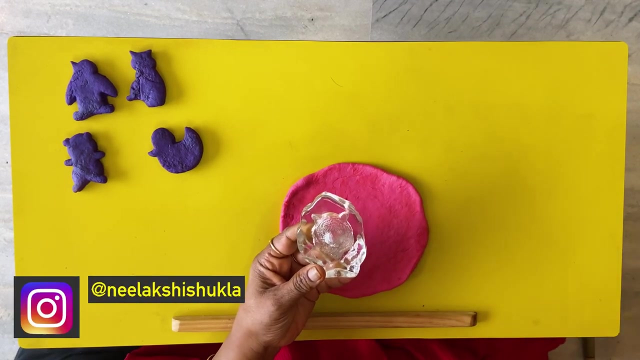 let's take pink color. let's see what do we have. I have some things I've just picked up. you know, just looking around the house so I have tiger here and I have Jesus in Jesus Christ. so let's see if I can put this mold put. 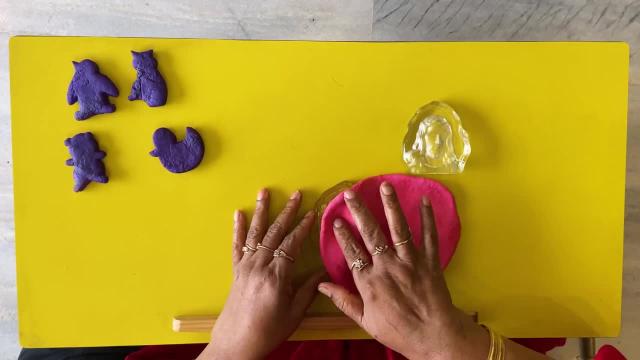 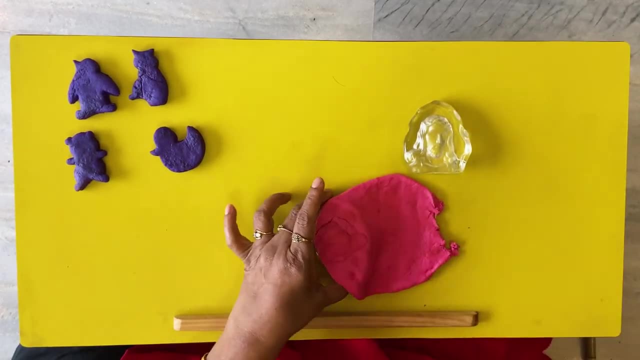 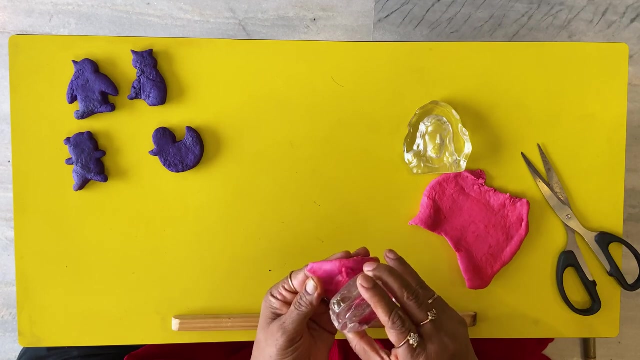 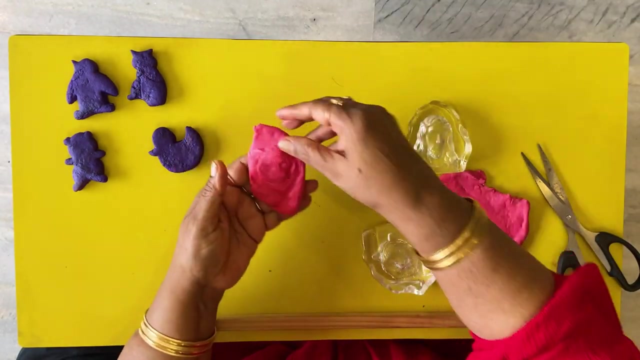 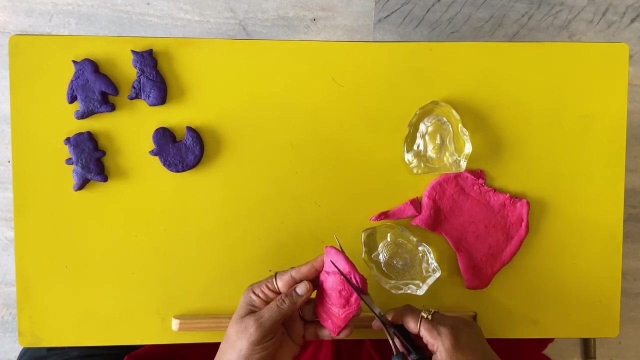 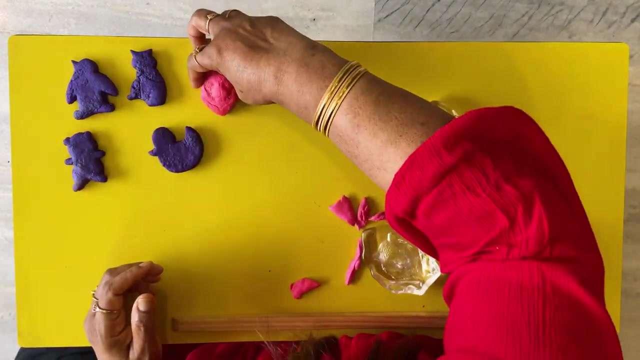 this inside the mold? do I get an impression? let's take it out and see what we have. Wow, here we have a mermaid. have a tiger. if you want, you can cut out the rest to give it a shape. if your children are bigger, children will love to see the sudden impression that is there on their door. 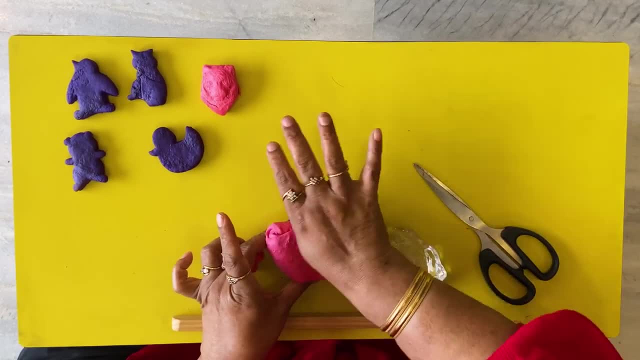 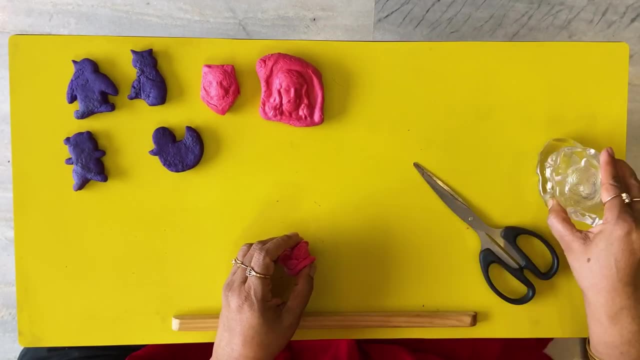 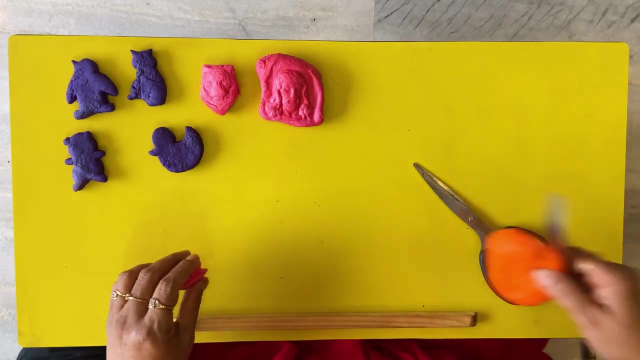 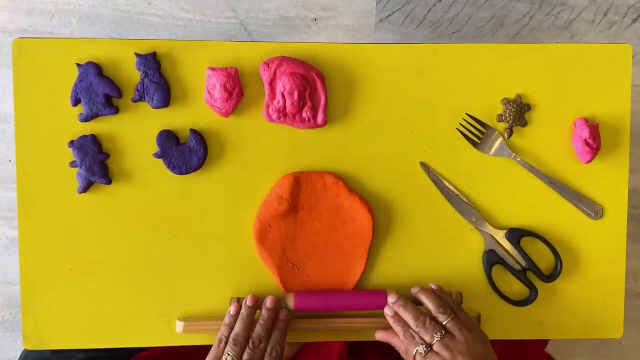 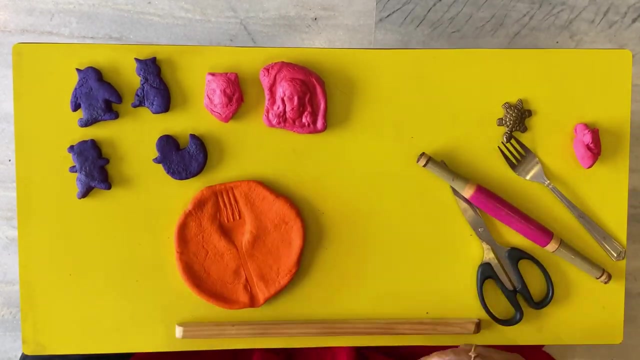 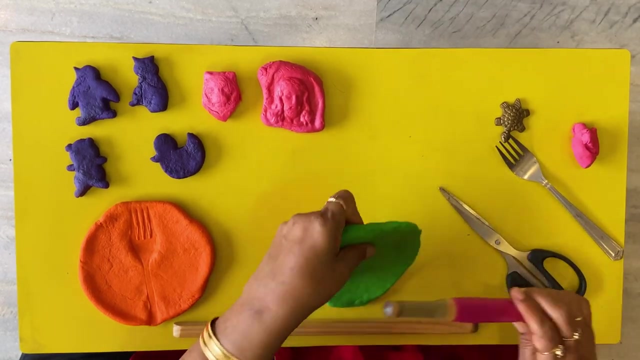 so here we have jesus christ. now you can pick up random things from your house to do this. so i took a fork. also, here we have a fork. let's see what i can do with the fork. so you can teach them colors. you can tell them: get the purple dough, get the pink dough, make a pink. 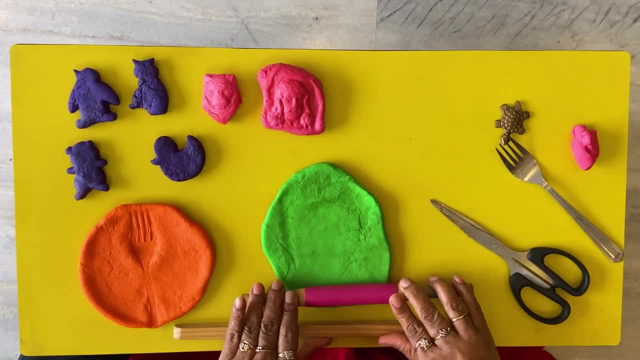 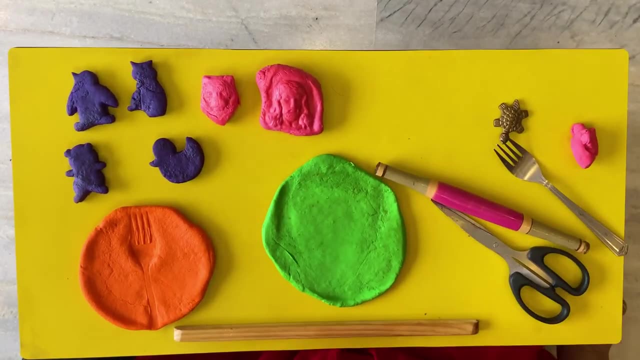 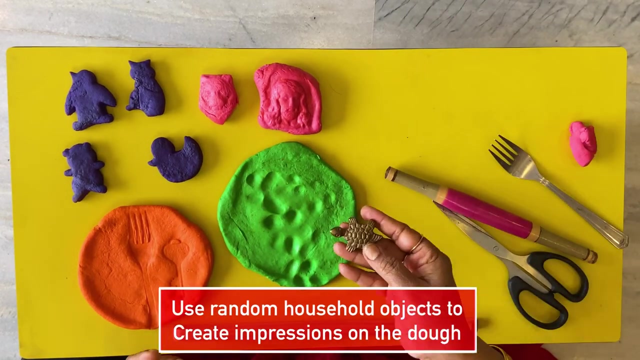 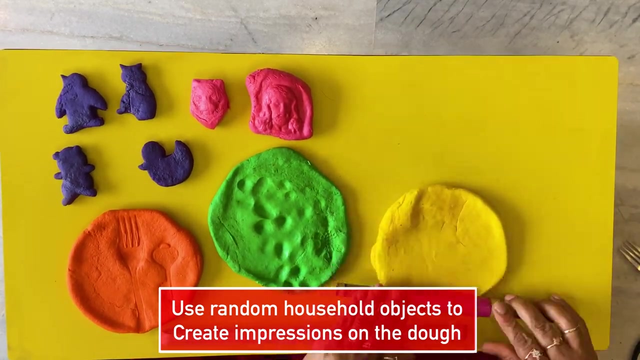 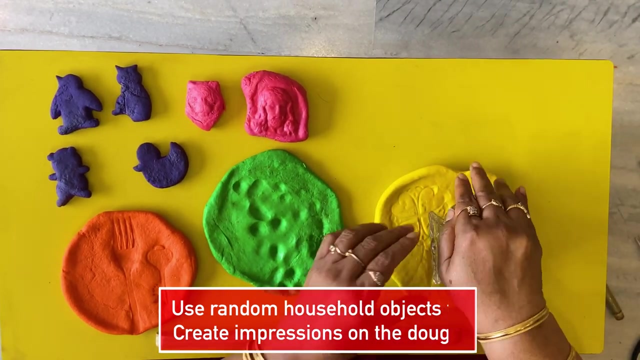 jesus, make a pink tiger, get the impression of the fork on the orange dough, and so on. so this is what it looks like when it's done. so i used the mouth piece like this. so we continue like this with all the household items that we have. 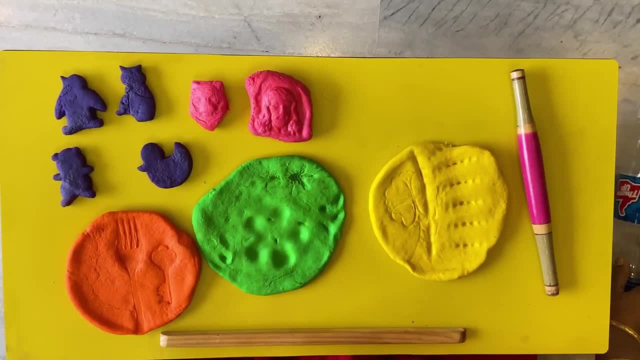 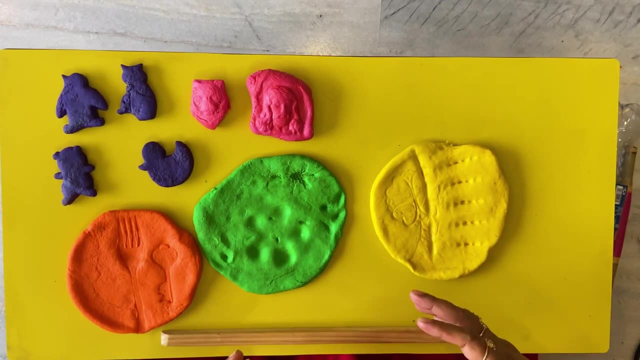 and we can keep on making impressions. so that's it, and you can let your imagination go wild and use anything that's available in the house and just have fun with the dough and any idea with this specialty. we can do everything that we wanna do with this. say: just take your. 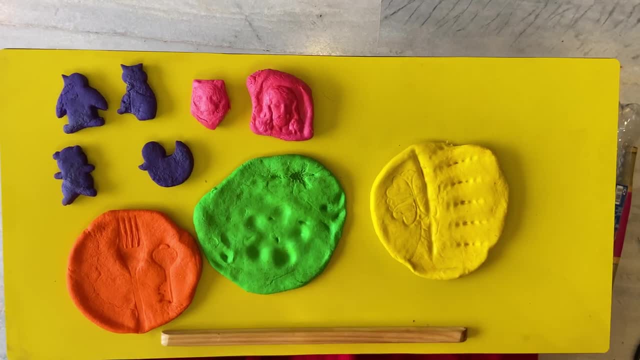 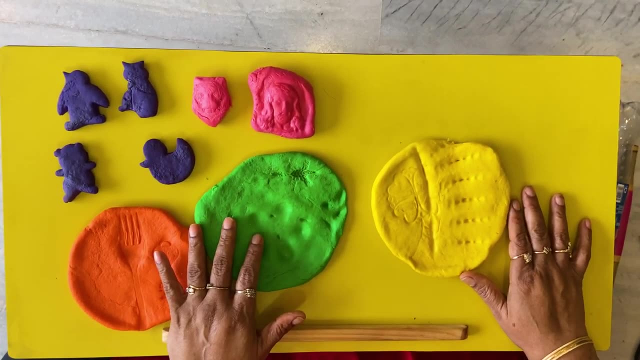 acrylic sugar powder, iron and pour the vezes, circa few drops justuto. we did all these things for this group of children can do this from 1 years to 6, 7, 8, 9, 10 years, it doesn't matter. the end of the child the more creative and you know you can think of.